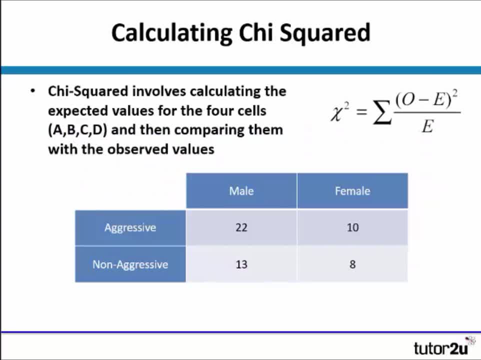 inmates in a high security unit. So chi-squared involves calculating the expected values for the four cells here in the table and then comparing them with the observed values. So we've got some nominal data. so aggressive and non-aggressive behaviors for male and females. 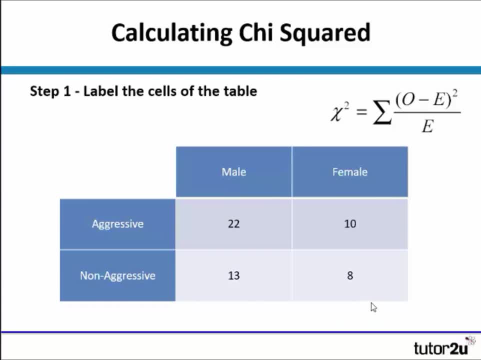 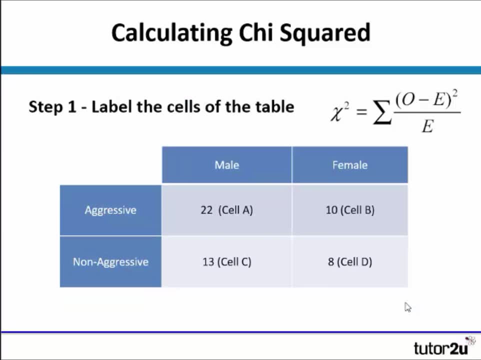 So the first thing that we do in chi-squared is label the cells. This just helps us with our calculations And we don't give them fancy names like Bob or Jeff, we just give them names. We give them cell A, B, C and D, And this is quite a small table, but you could have many. 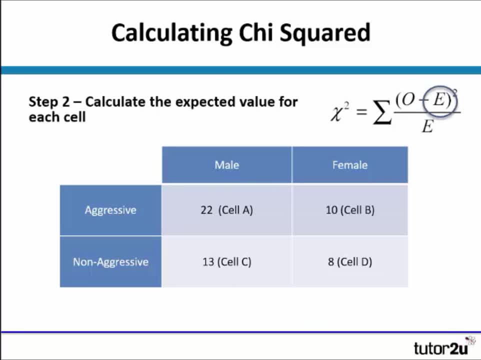 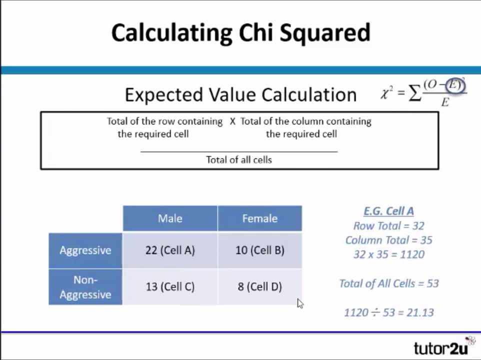 different variations as well. So cell A, B, C and D. So, if we look at the formula, the thing that we need to do is calculate the expected value for each of these four cells, And the way in which we do this is finding the total of the row containing the required cell, And then we find the total of. 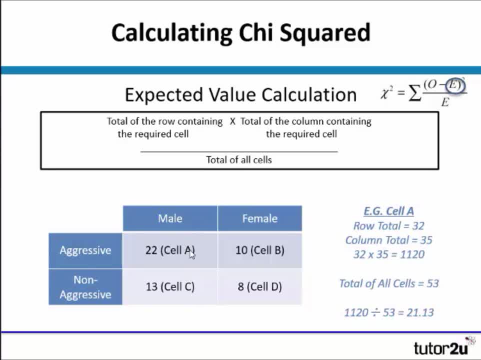 the column of the total of the column where the required cell is, And then we divide it by the total of all columns. So I've given you an example here for cell A. So our row total would be 22 add 10,, which is 32.. And the column in which cell A is is 22 add 13,, which is 35.. We then 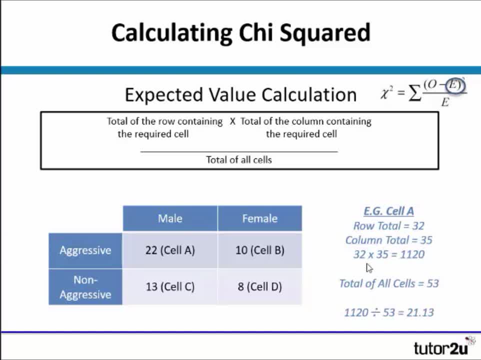 as you can see from the formula up here, times those two together, So 32 times 35, by my calculations is 1,120.. If we add up all the four scores, this gives us the total of all cells, So 22 add 10,. 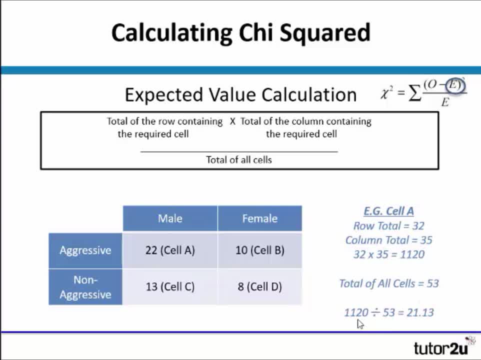 add 8,, add 13,, it's 53. And then we divide the original answer of 1,120 by 53, which gives us an answer of 21.13.. And we have to do this for all the other cells. Okay, so I've given you the row. 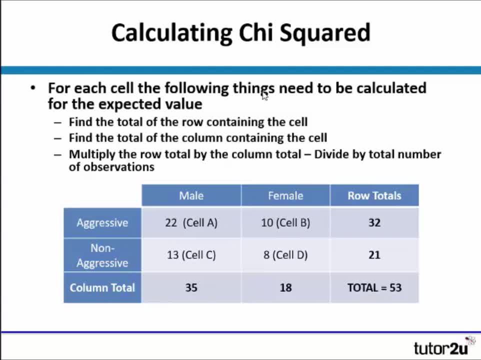 totals and I've given you the column totals and hopefully that will clarify the steps. So we always need to find the total of the row and the total of the column containing the cell And then we divide that by the total number of observations. 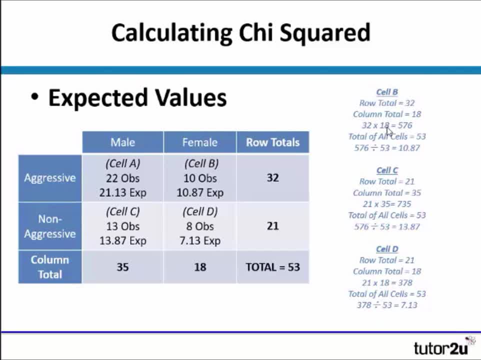 So here we go, cell B: I've done the same calculations And all I've done here. in the table is said what our observed value was, which was the original data in the table, and then given you the expected value as well. Okay, so we've got 10.87,, 13.87, and 7.13.. 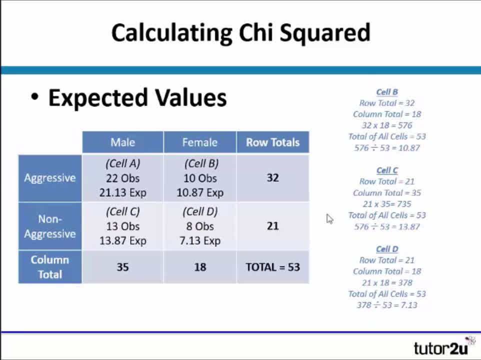 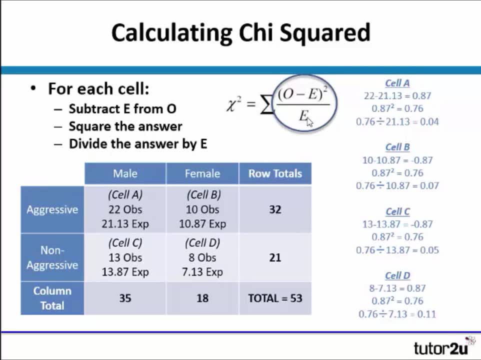 And all the calculations are there and feel free to pause the presentation and to have a look at those in a bit more detail. So now we've calculated the total of the row totals and we've got the total of the row totals and we've got the expected value. This means that we can complete the rest of the formula. 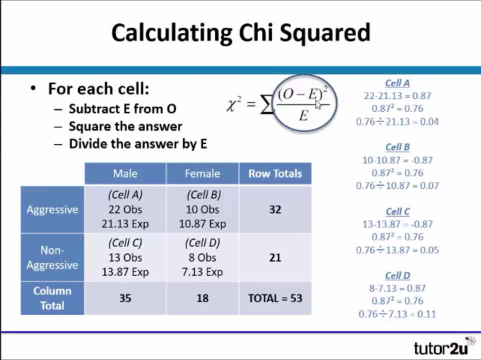 So for each one, what we need to do is subtract E from O and we need to square that answer and then divide it by E. So here we have, for cell A, 22 minus 21.13, which gives us a result of 0.87.. 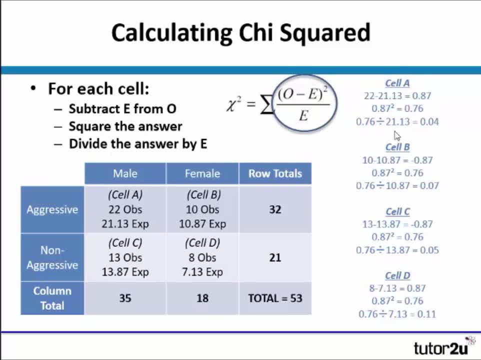 We then square that, it gives us the answer of 0.76.. And then we divide that by the expected value, which is 21.13.. This gives us the answer of 0.04.. And again, as you can see, I've given you the calculations for cell B. 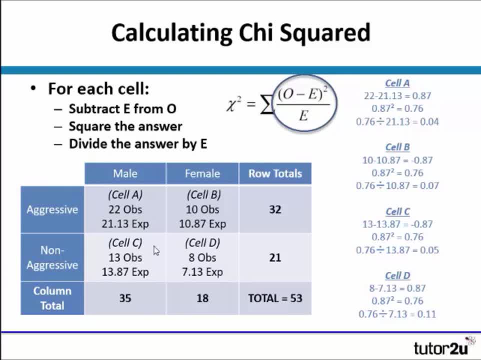 C and D as well. They all follow the same idea, And that's why it's really important to label your cells and also keep an eye on what's your observed value and what's your expected value. So if we just look at cell D, for example, our observed value is 8.. We need to take away our 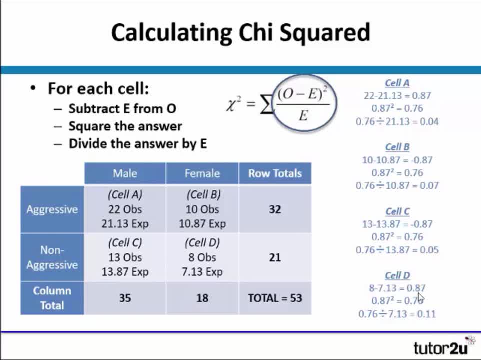 expected value, which was 7.13., Gives us the answer of 0.87.. We then need to square that answer and then divide it by the expected value of 7.13. And that gives us the answer of 0.11.. The next step, the final step, is quite easy. 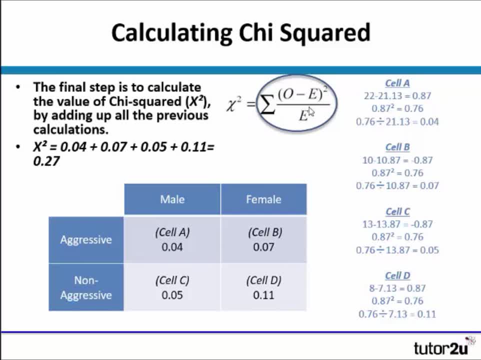 All we need to do is calculate chi-squared by adding up all those values from our previous calculations. So I've left the calculations here and we add them up. So 0.04,, 0.07,, 0.05,. 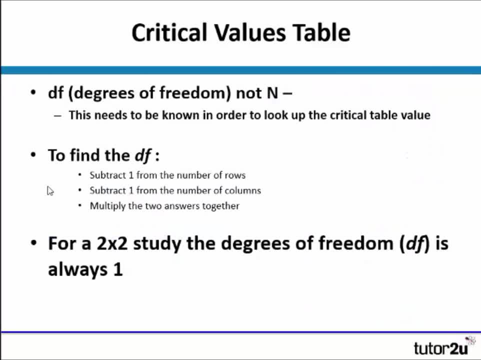 and 0.11 gives us 0.27.. So we need to bear that one in mind. But before we get there, we need to also think about our degrees of freedom. So to look up our values in the critical value table, we're going to look at our degrees of freedom. So what we're going to do is we need to say: 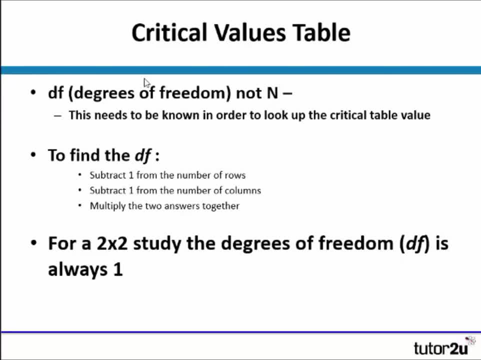 which is the first value below The second value on the second measure. So if we look up the values on the second measure side, that means table. we're not going to be using n for number of participants. instead we're going to look at degrees of freedom, and so degrees of freedom is calculated by. 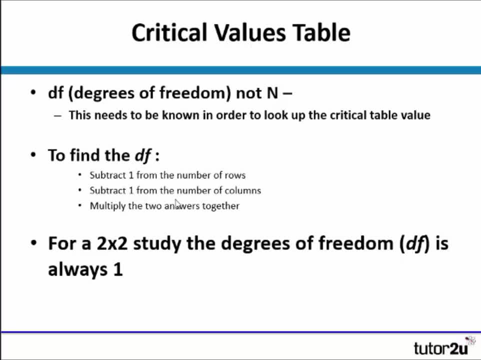 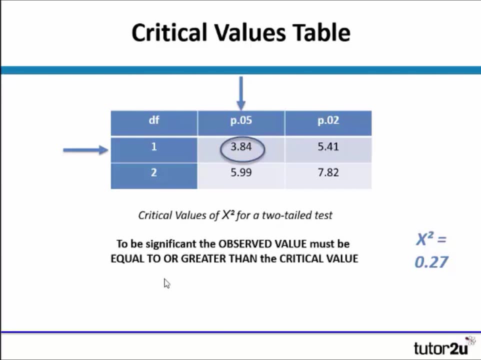 subtracting 1 from the number of rows and subtracting 1 from the number of columns and then multiplying those two answers together. so for a two by two study like the one that we're conducting, the degrees of freedom is always 1. 2 minus 1 is 1. 2 minus 1 is 1. 1 times 1 is 1. so here we have a little bit of a. 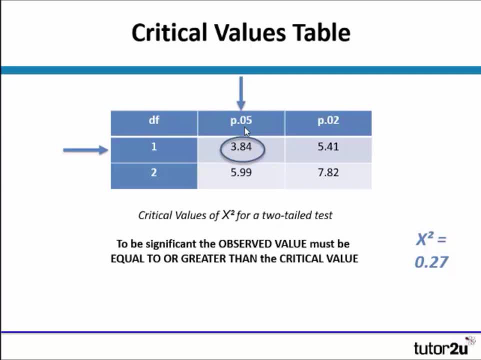 critical values table and we're looking at P, point zero, five. so the probability of our results being huge chance is less than five percent. our degrees of freedom is one and the answer that we find in here is point zero, three, point eight, four. so be significant our observed value. so the thing that we have 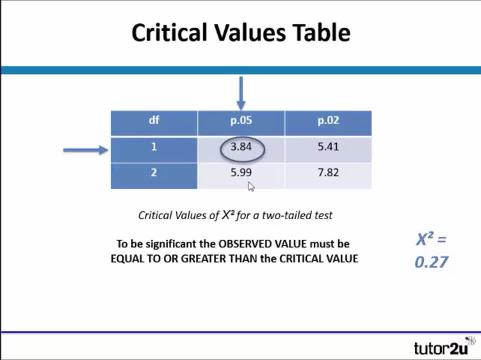 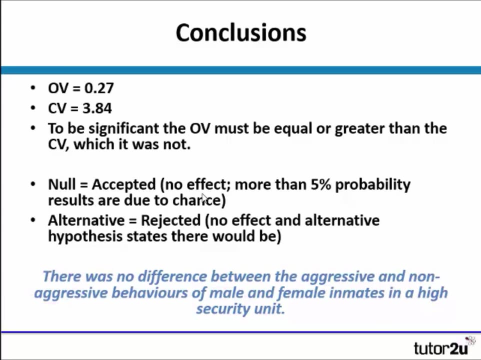 calculated must be equal or greater than the critical value. so that's the information in the table. as you can see, our poor little chi-squared calculation of point two seven is not bigger than point three two 0.84.. So that means that we are going to accept our null because we haven't found an effect. and 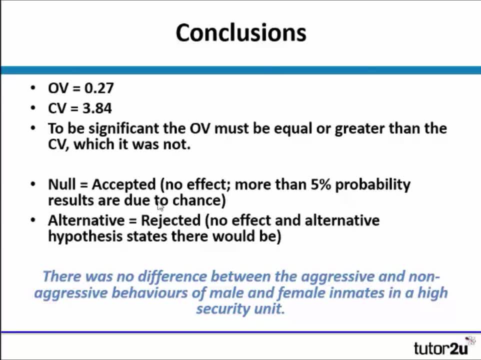 there's more than a 5% probability that our results are due to chance. Because we've accepted our null, we're going to reject our alternative, because this experiment, this study, found no effect and our alternative hypothesis states that there would be. So, overall, in conclusion, there was no. 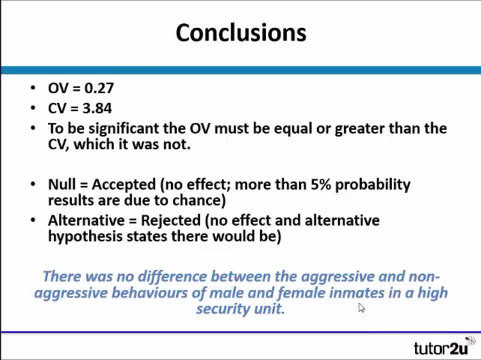 difference between the aggressive and non-aggressive behaviours of male and female inmates in a high security unit. That was a brief outline of chi-squared for A-level and IB psychology. 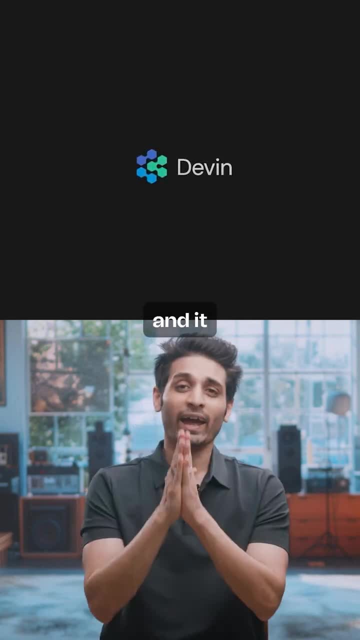 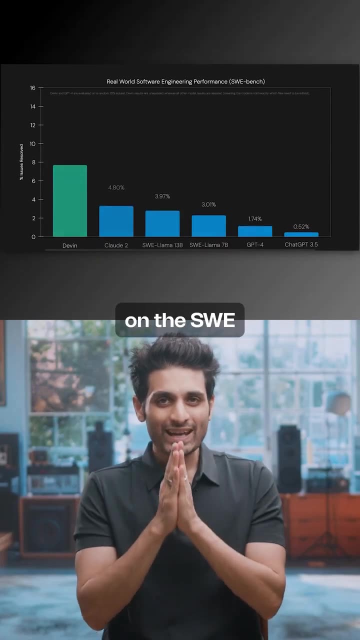 A new AI tool was released recently, called Devin, and it scared the holy ghost out of software developers all over the world. Made by Cognition Labs, Devin is the new state-of-the-art on the SWE Bench coding benchmark and successfully passed practical engineering interviews from leading AI. 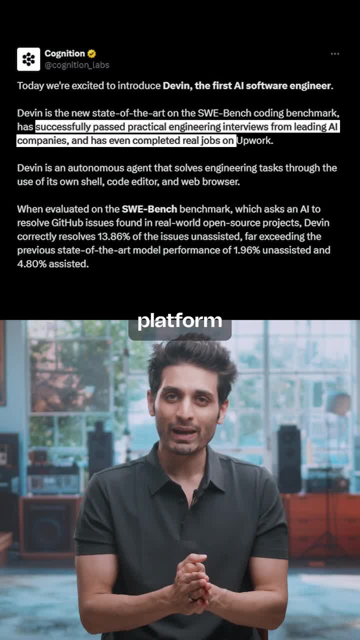 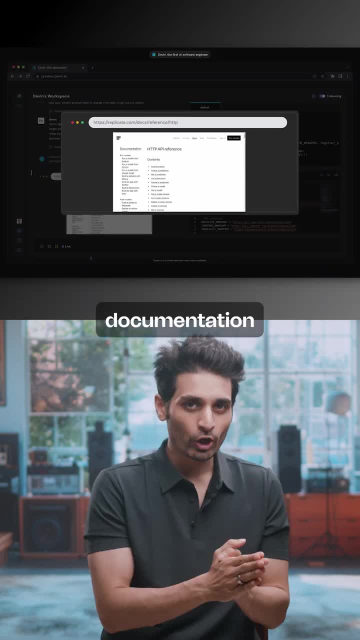 companies and even completed real jobs on the freelancing platform Upwork. Devin can solve problems in unfamiliar technologies that it has no exposure to, which means it can read documentation and make decisions. It even writes tests for you. Devin is not actually foolproof. 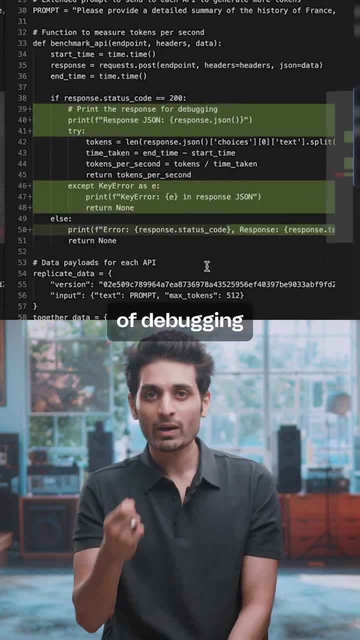 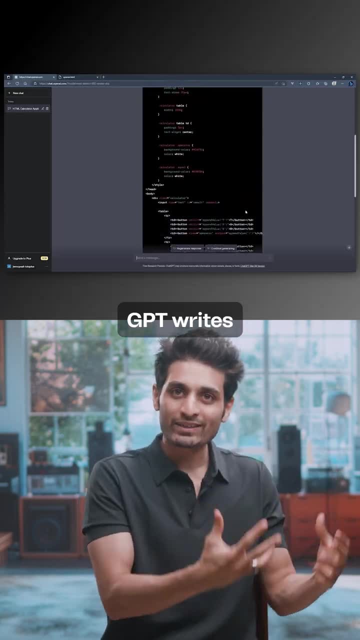 It does make mistakes, but it's also fully capable of debugging the code. Also, if you give it a GitHub issue and the code base, it can get to solving it. And we do know GPT writes code. but why doesn't it make full apps properly yet? Well, that's because GPT has ADHD. It has 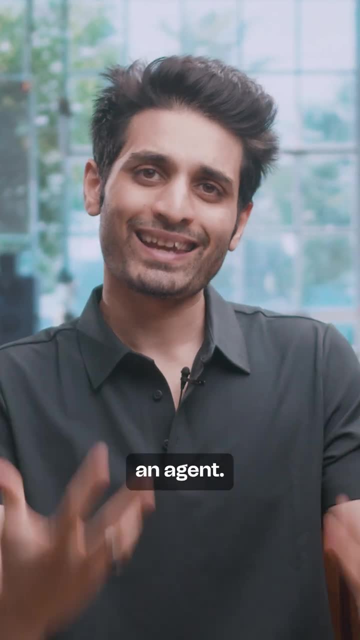 attention deficiency and it constantly gets sidetracked when you use it as an agent. If Devin has actually solved this, there are far more implications than just code, And it also means that it can be used as an agent. And it can be used as an agent. And it can be used as an.